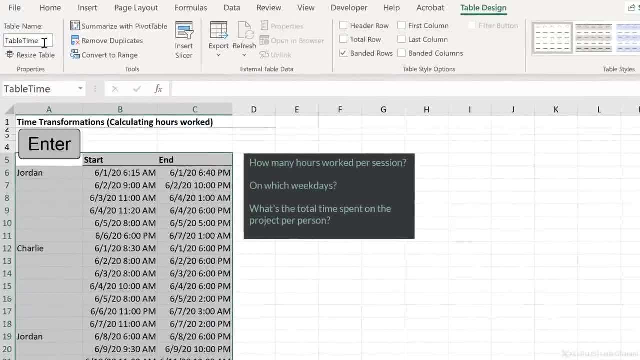 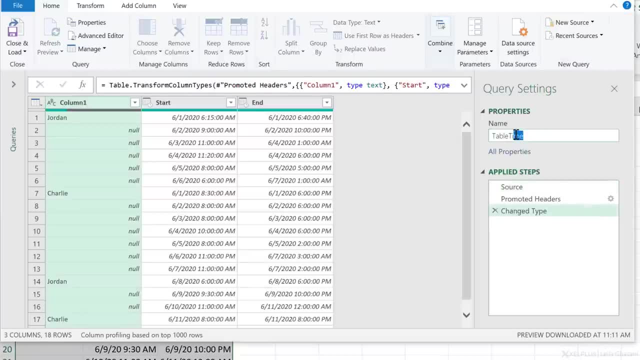 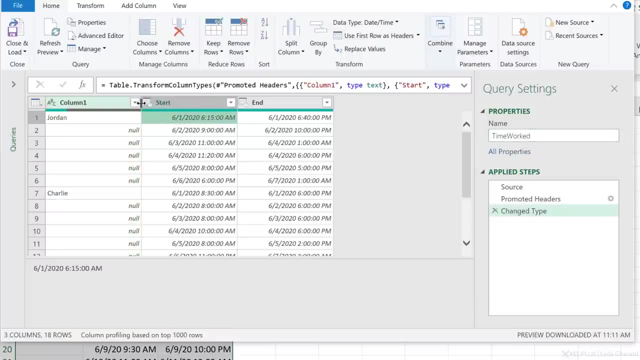 Call this table time and enter. Now let's send this to Power Query from table range and call the end result. time worked Now the date and time here was recognized properly. The first column doesn't have a name. I'll give it the name: name. 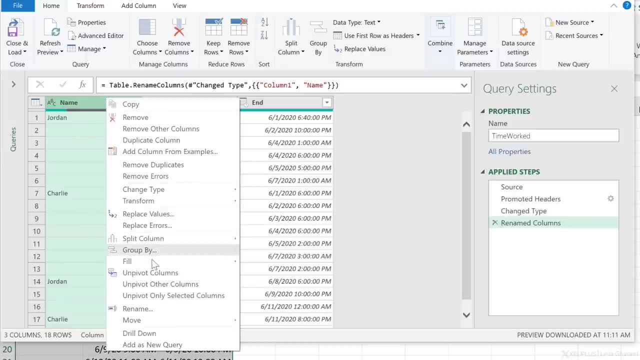 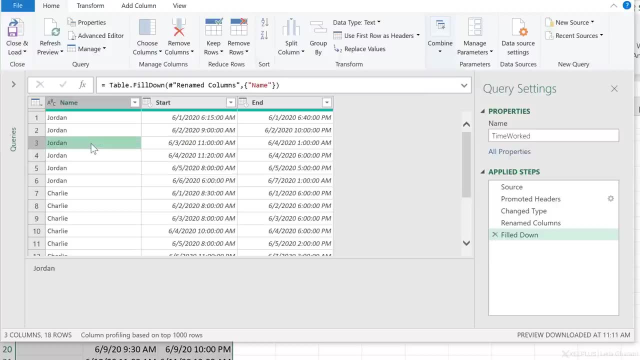 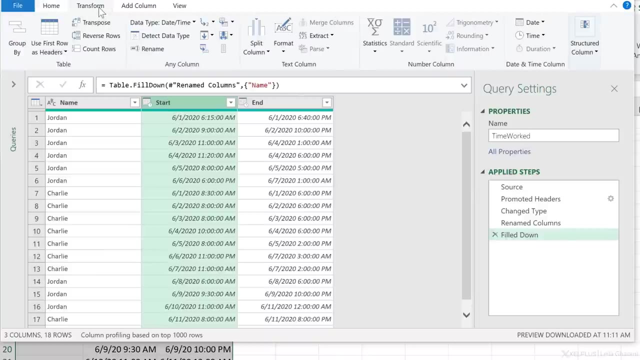 It would make sense to send these down, So let's right mouse click fill. send these down Now. each row or each record here is associated with a name, As we saw before. with date transformations, you can find the time transformations either. 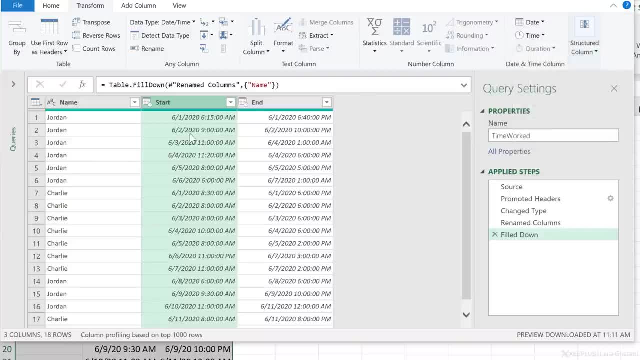 in the transform. So I'm going to add a new column right here. So if you actually want to change this to something else here, you would directly make your selection in the transform tab, Or if you want to add a new column, you'd go to add column and make your selection from here. 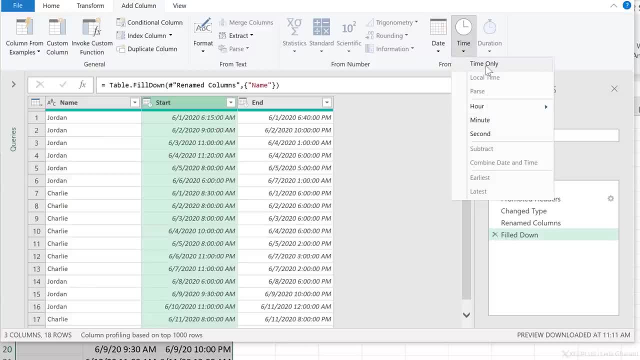 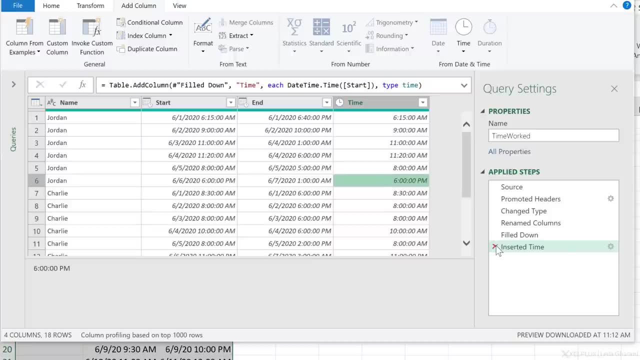 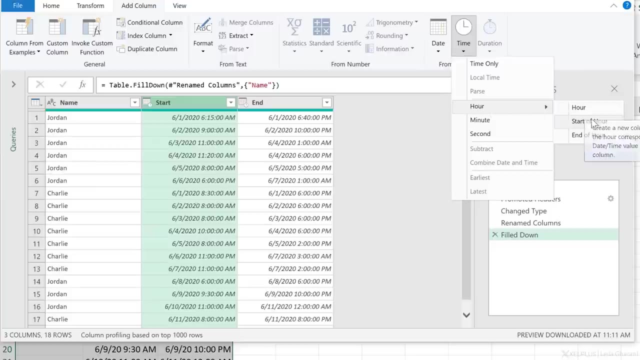 So I'm going to keep this as is and add a column. If, let's say, I wanted to strip out the time, only I can select this. That just gives me the time portion of my original value Under hour. we can strip out the hour. 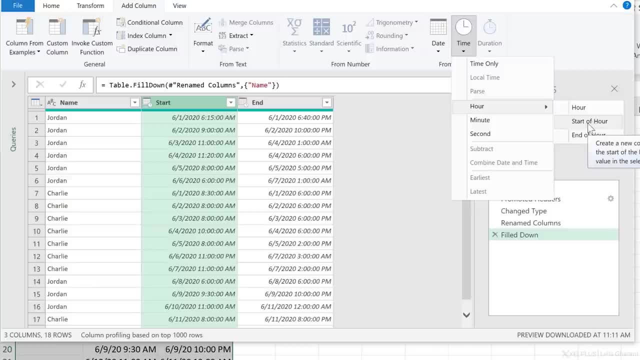 We could also strip out the start of the hour. Notice that sometimes the work is started at like 6.15,, 11.20, and so on. So if I go with start of the hour, I get the same type back. 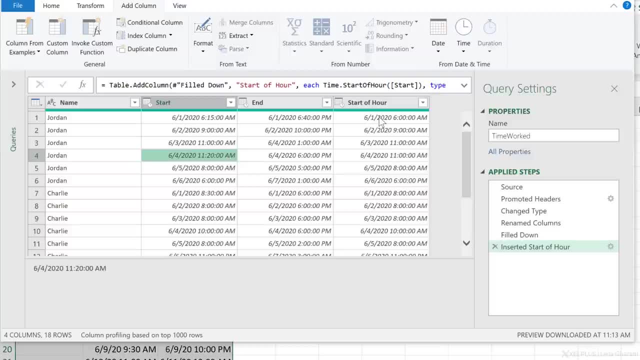 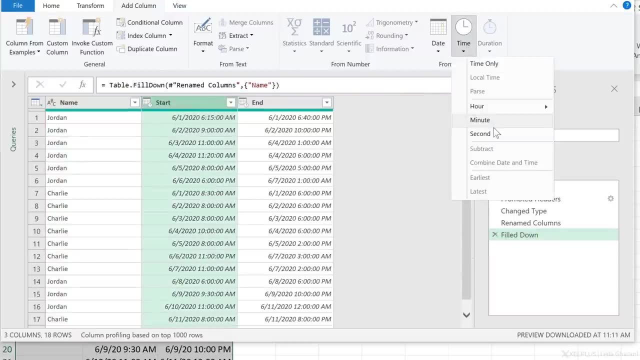 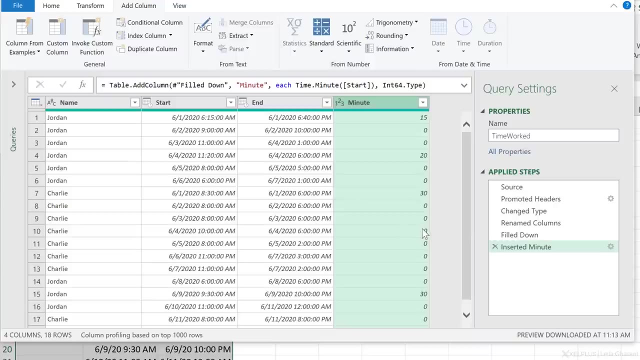 but I see 11 instead of 11.20, and six instead of 6.15.. Now, in addition to these, you can also strip out the minute or the second of this time. So, for example, if I go with minute, that's what I get. 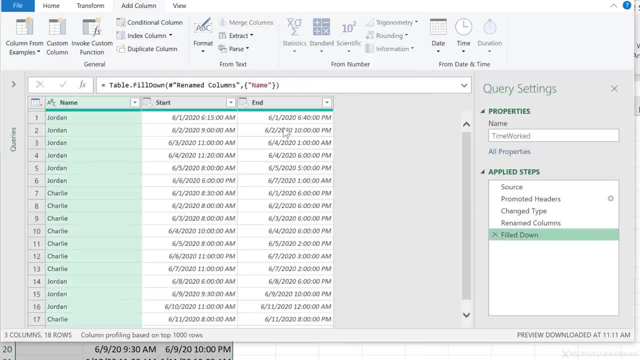 Now let's go back to the original questions that we had to address. We wanted to calculate how much time each person spends per session. Now, under time, notice that there is an option to subtract, but it's grayed out. That's because we need to select more than one column. 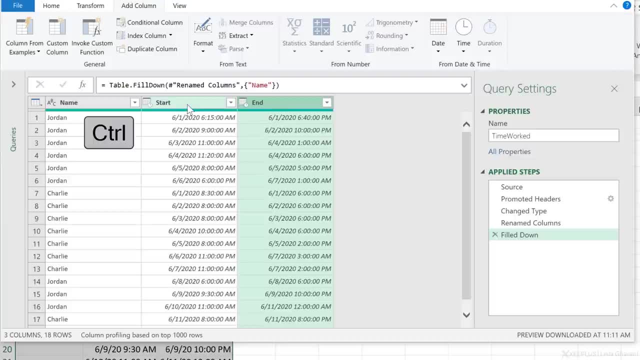 So I'm going to select the one I want to subtract first and then hold down control. select the second column. Now it's not grayed out anymore. When I click subtract, I get a duration back. Remember, duration is read in this way: 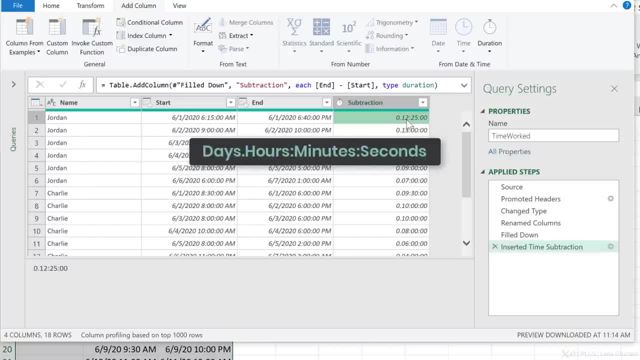 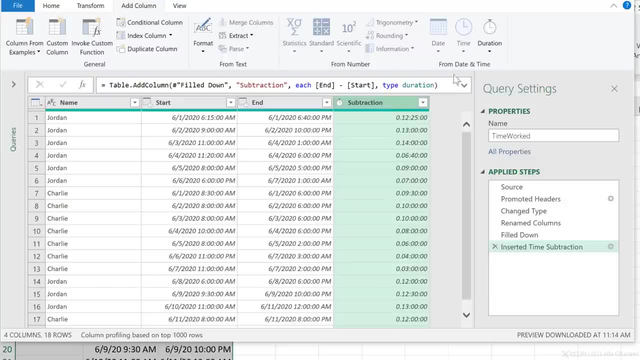 that the first number here is associated with the number of days, hours, minutes and then seconds. It would make sense to get this back in the number of hours. So let's go now to the duration options, and I could make my selection here. 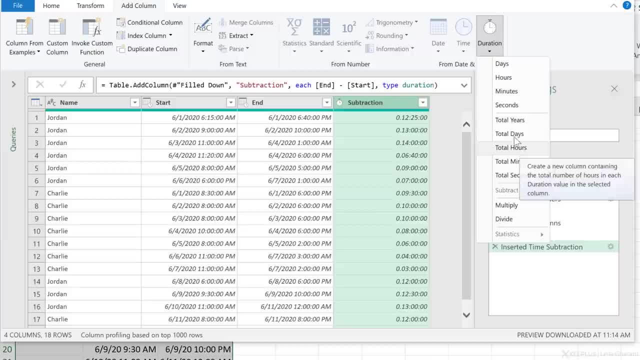 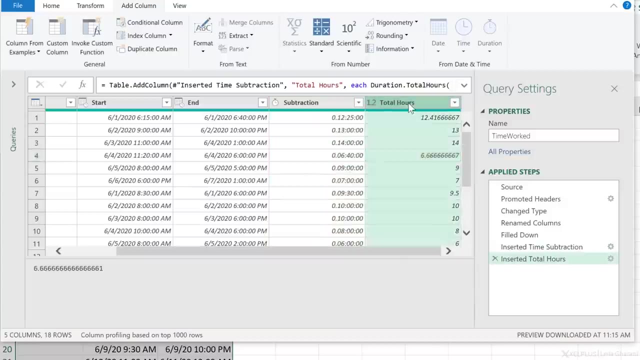 But notice, I have hours and I also have total hours. The difference is this: When I select hours, I get everything rounded up. If I go with total hours, I get the exact hours. Now let's round these. Select the column. go to transform rounding. 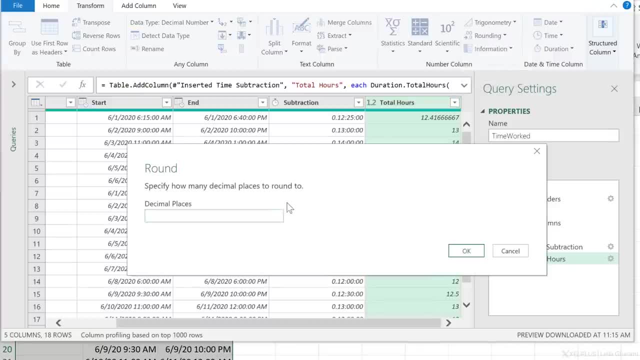 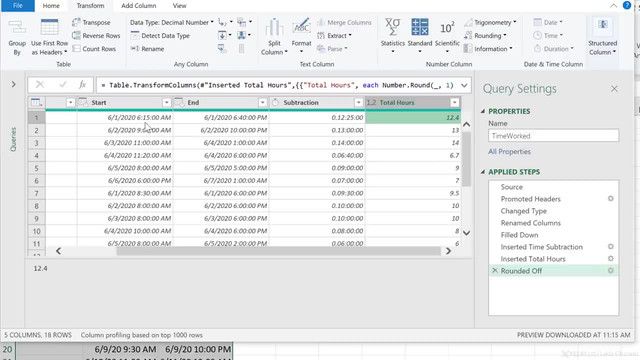 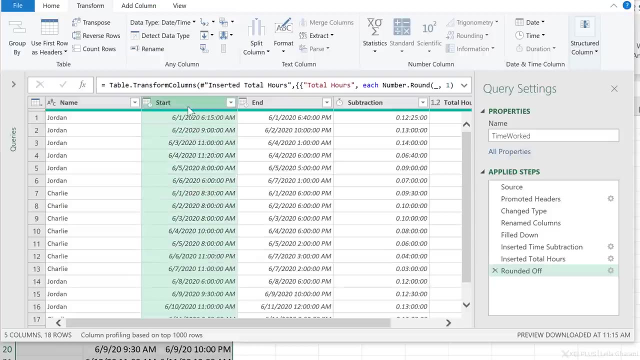 Now we could round up or round down, but let's round these this time to one decimal place and click on. okay, Now that's the total hours worked per session. Next thing we wanted to know was: on which weekdays do they work? So let's go and get the weekday name from the date here. 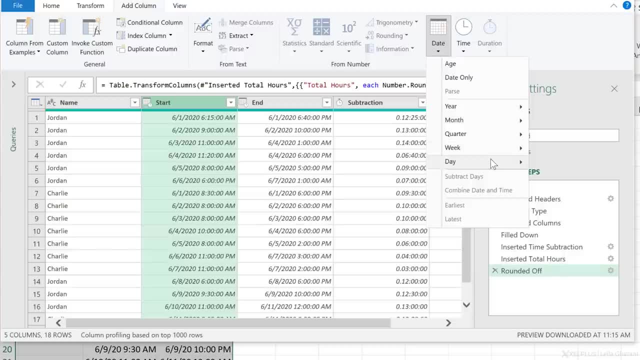 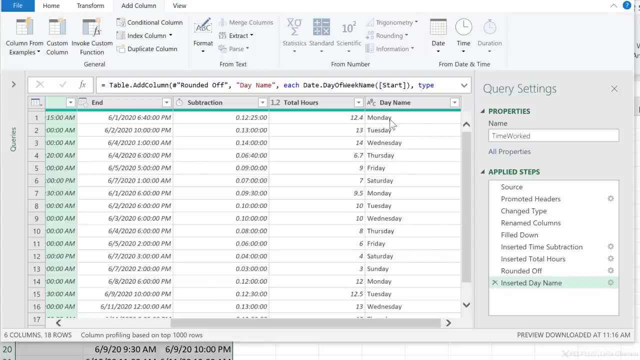 I'll add a column again this time Go to date, day and name of day. Now it would also be nice to have the name of the day, but also have the day number on the side here. so let's do that. 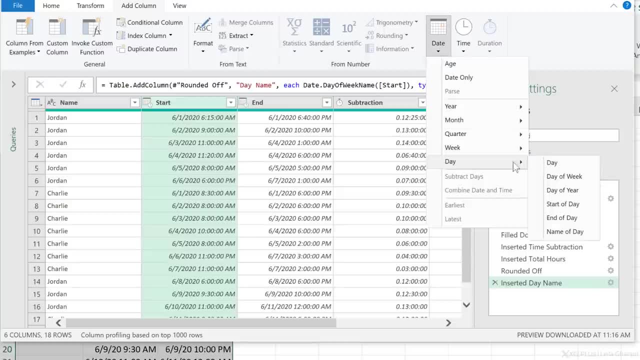 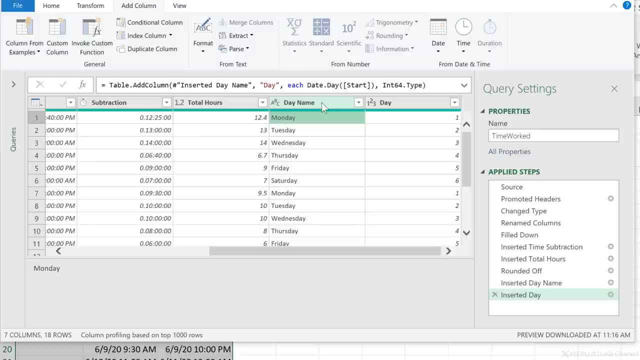 With this column highlighted. let's go back to date day, and this time just day, But it would be also good to have these in the same column, so let's merge them together. Click on the first one. hold down control. 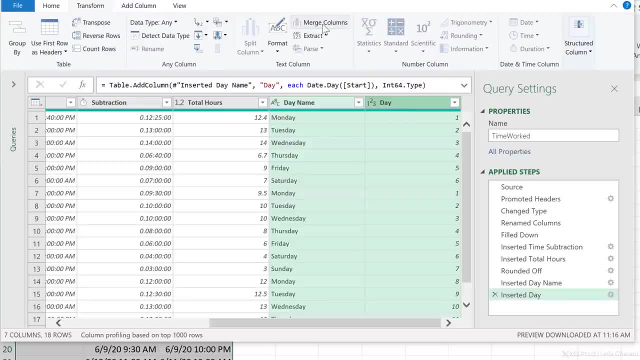 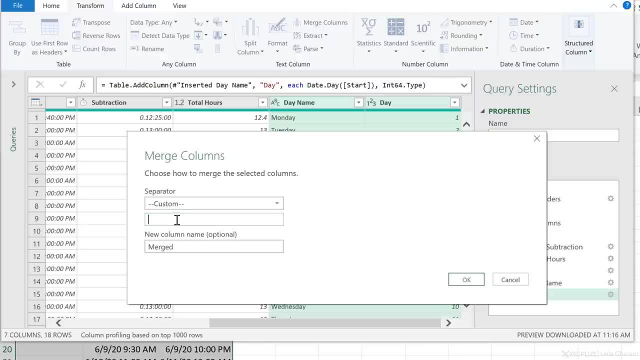 click on the second one, go to transform this time and merge the columns. I want to bring them together. For the separator, let's go with custom space slash and I'll call this workday. Go with, okay. and now it's easier for me to see. 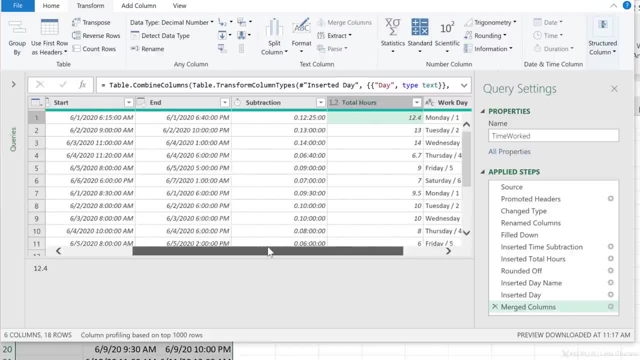 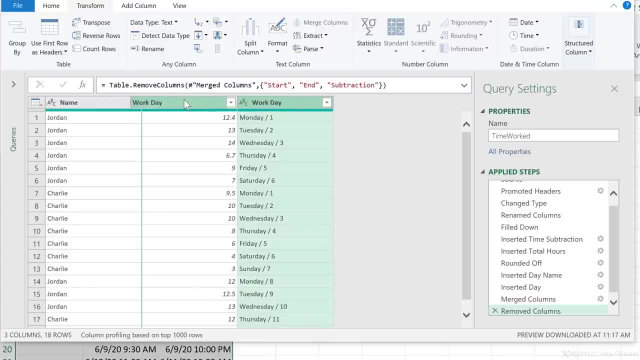 which day that date belongs to. So now let's remove what we don't need. Let's just highlight these, press delete, and I'm just going to rearrange these together and my report is done. Let's send this to Excel. 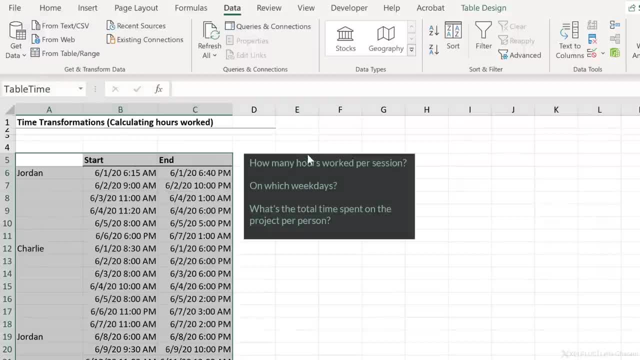 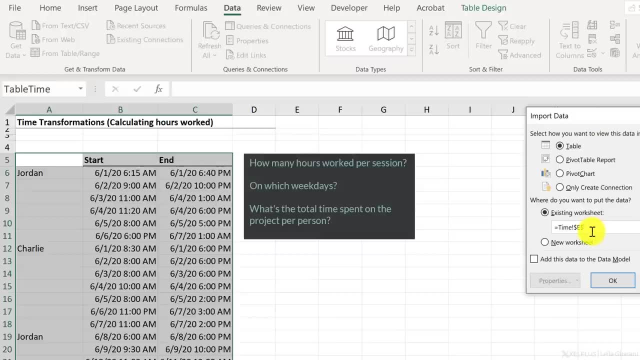 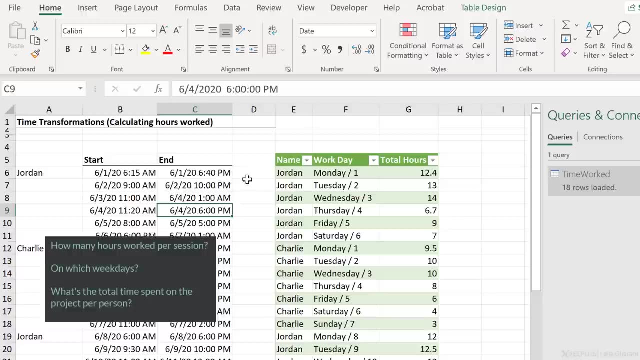 Go to home, close and load, close and load two Existing worksheet. let's put it on E5, and go with. okay, I'm just going to put this out of the way here, So this way we can easily see how many hours. 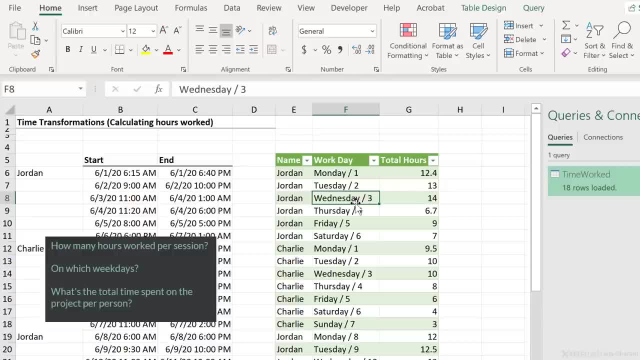 each person worked for each session. Now let's answer the last question: what's the total time spent on the project per person? Basically, I want to group these by the names. I'm not interested in the workdays, just these two columns. 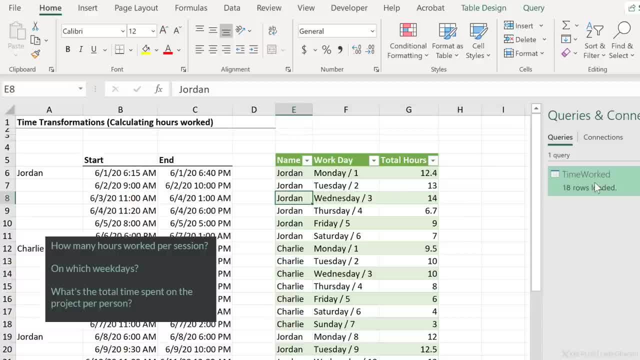 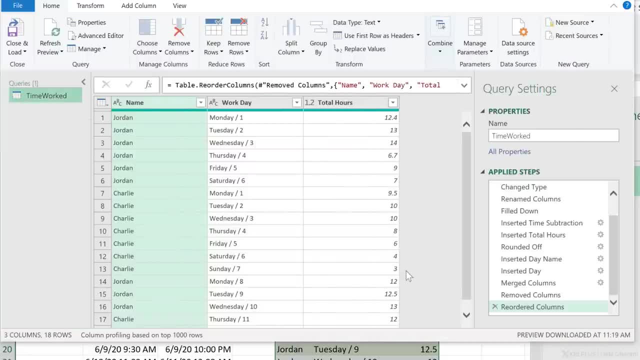 Now, since I'd like to keep these report as well, let's create a second query by referencing the first query, because my starting point is this query, which is the last step of this query. That's going to be my starting point, So I'm going to right mouse click and reference: 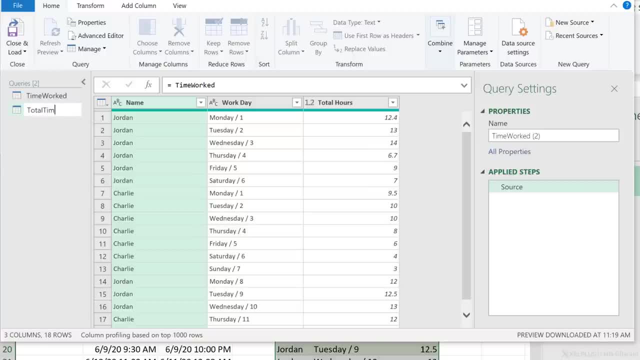 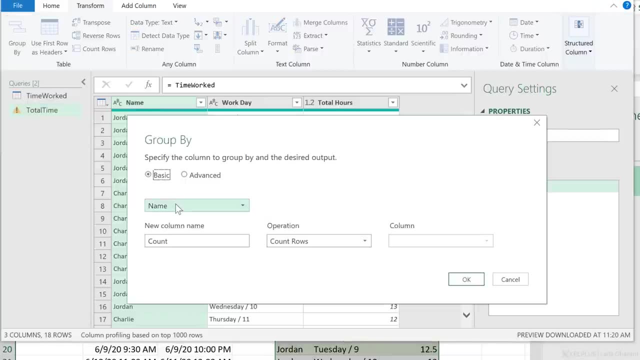 Press F2 to rename total time With the name column, select it. go to the transform tab group by. We're grouping by name. The new column should be called, let's say, time worked. What we want to do is get the total. 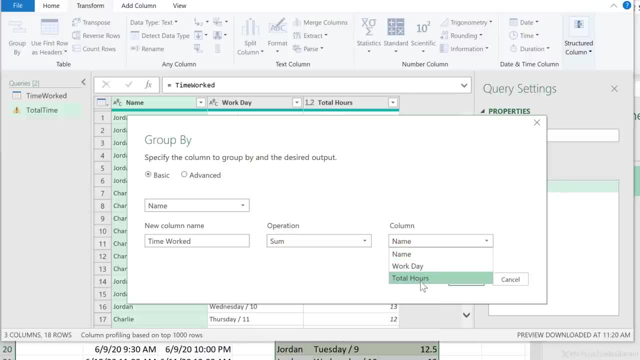 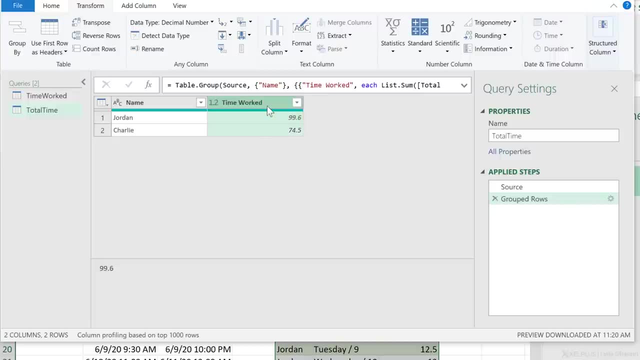 so we want to add up the total hours here, So let's switch this to total hours and click on. okay, Now I have the exact hours each person worked on the project. It would probably be nicer to round these from the transform tab. Let's go to rounding and this time let's round them up. 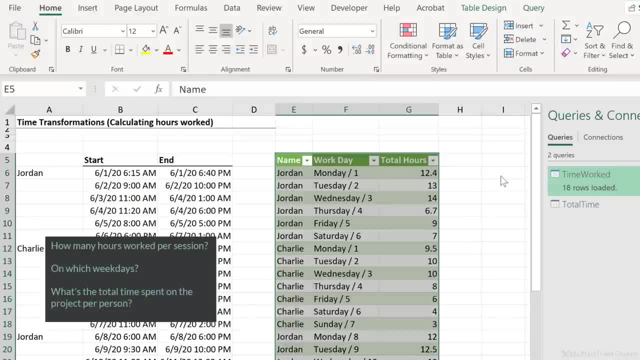 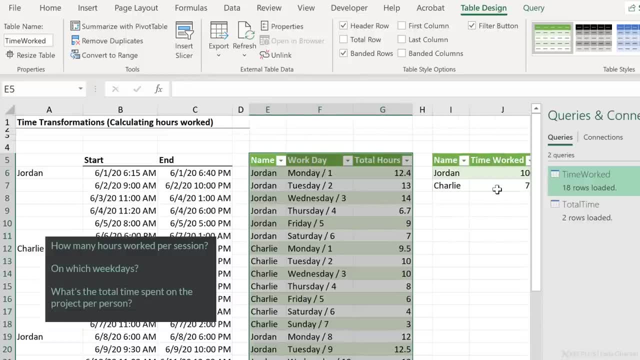 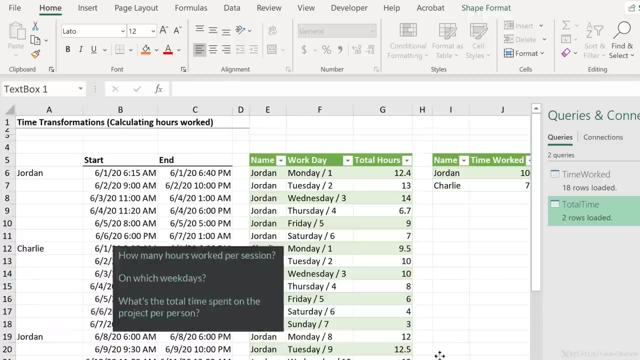 Okay, let's send this to Excel. close and load. close and load two And let's put it right here. Okay, so let's see who worked the most. Jordan spent 100 hours so far on the project. Okay, so now let's just move this out of the way. 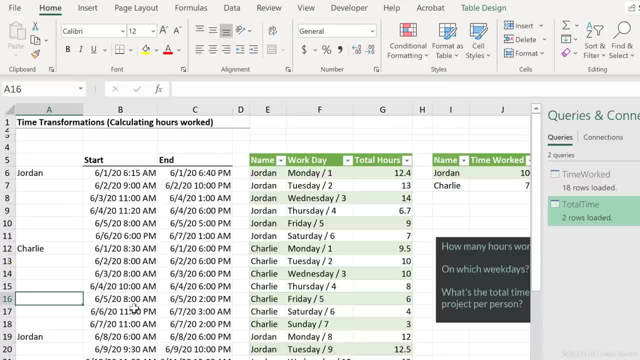 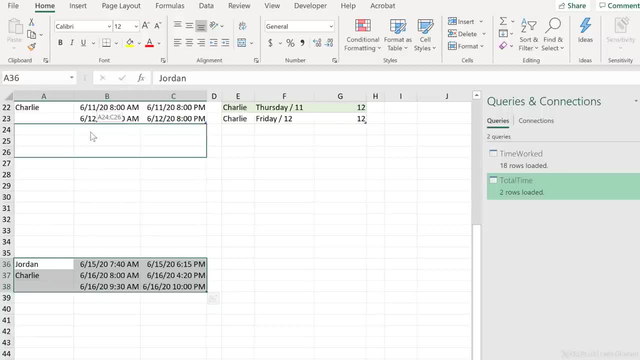 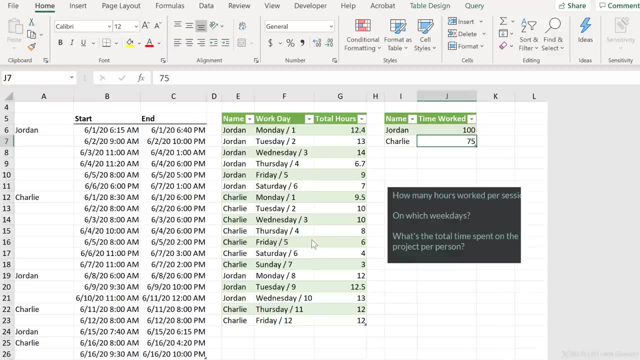 Let's see if these update when they continue to record the time spent on the project. So I have some sample data here. I'm just going to drag it and drop it inside the table. So we are going to refresh both queries and see if they update accordingly.